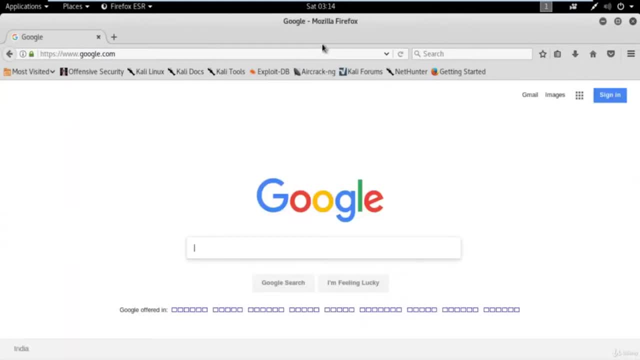 sample website. we will not attack on any live website, so it will be illegal if you try on somebody else website, right? so just you can try on your website. otherwise you can try on sample website. so the sample website I'm taking is onewebcom, because this is a sample website provided by Acunetix tool. so 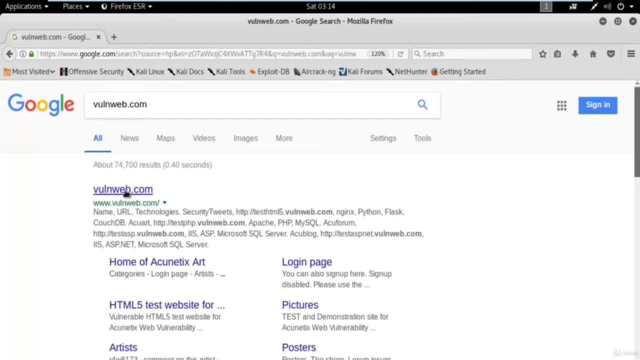 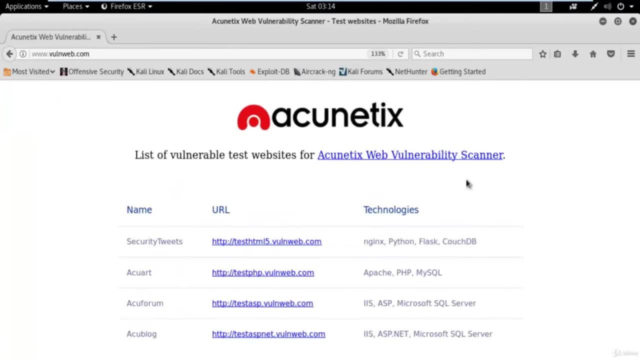 this is onewebcom and if you open this, this is the link of the website. open that, and here you can see on the screen. let me zoom it so that you can see on the screen. there are four links available, right, as we are working on MySQL, right? so I will choose the second one. 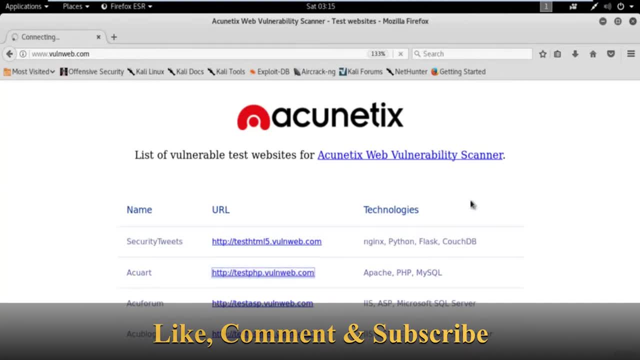 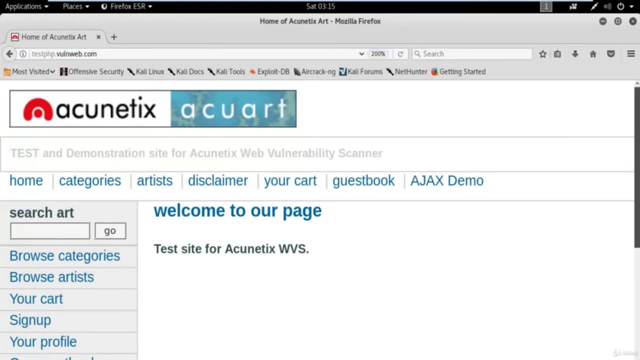 which is testphponewebcom. so click on that and open this website. so this is the website you can see on the screen right- testphponewebcom- and we will try to find out information about this website. we will try to find out. 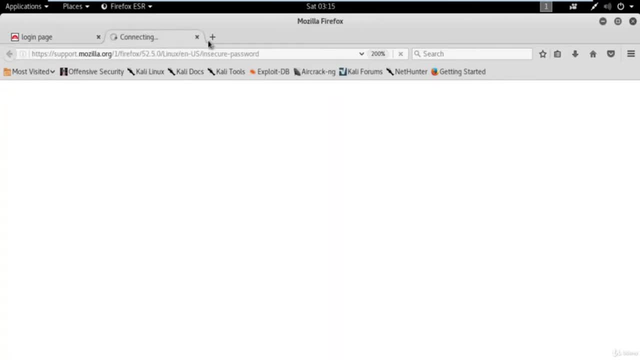 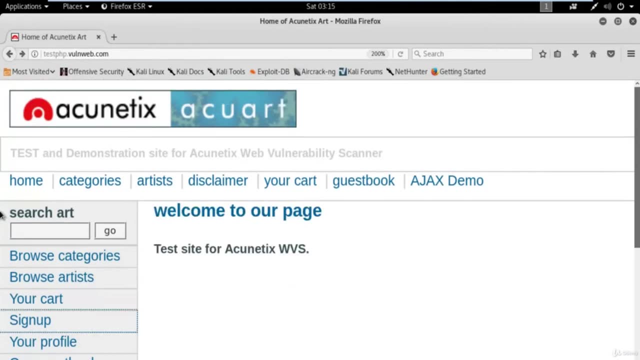 information about the username and password so that we can put here and get information about their database etc. right, so how we can attack on this website? first of all, to attack via SQL injection, you need to find the link of the website that that is really important to. 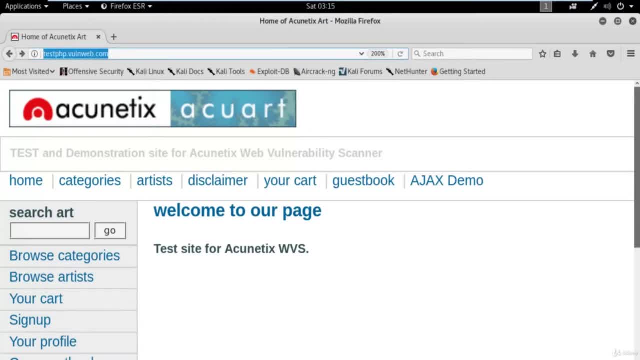 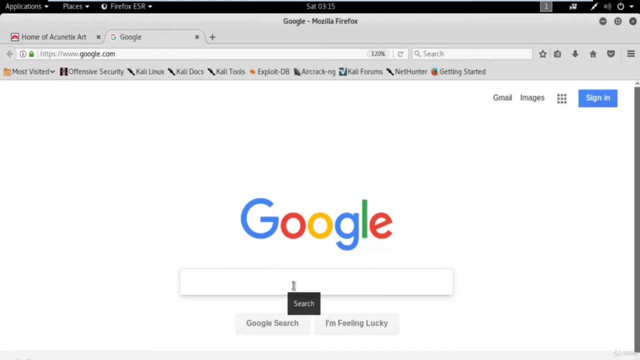 start. so how you can get the link: just copy the URL area here right. open a new link, open a new tab, actually, and here you can simply type here: site colon. paste the web URL here, space PHP question mark ID equals to right. it will help you to. 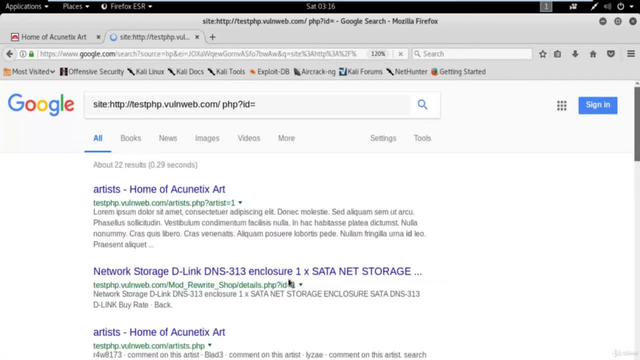 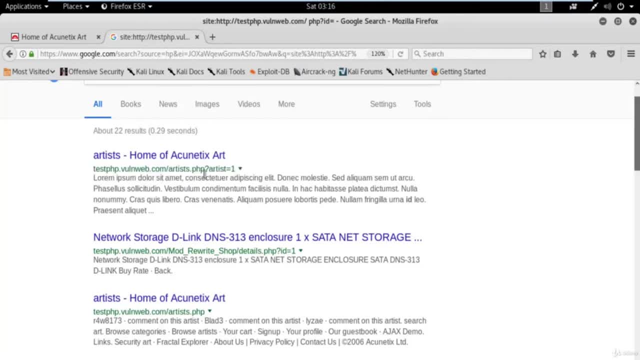 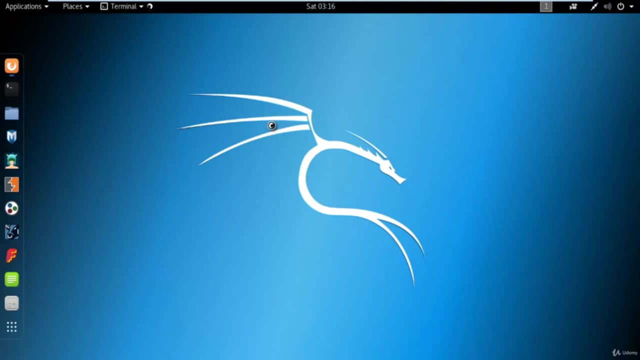 attack on the website testphponewebcom. slash artist dot. PHP question mark: artist equal to one. so let's take this link, copy that right and minimize everything. now do one thing: just open your terminal of Kali Linux operating system. let me zoom it for you. 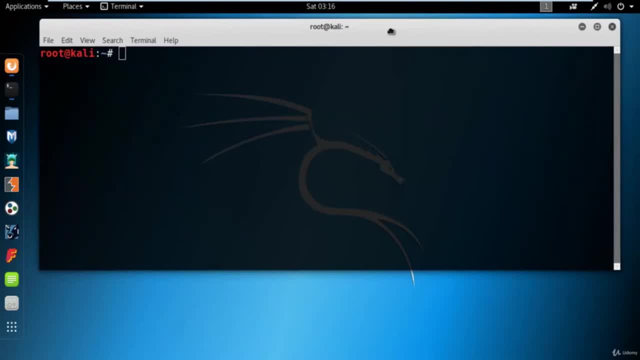 So we need to find a webdev database, database first of all, then later we will find out the table name, then column name and then the data, actual data which is inside the database. so my aim is here, the databases, so that we can move further. so how we can get the database name here, let me show you. 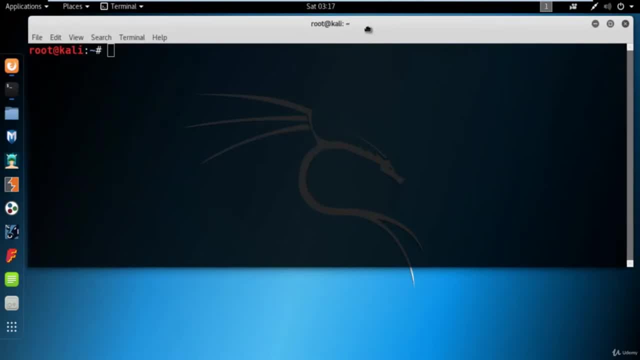 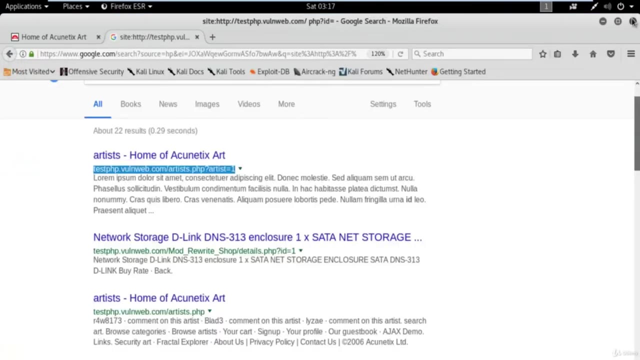 so there are some uh fixed commands available in sql map tool that we can use. so what you can do, you can simply type sql map space dash small u and paste here the link which you have copied from here and, uh, you can minimize this. all right, test php dot one, web dot com. slash artist dot php. 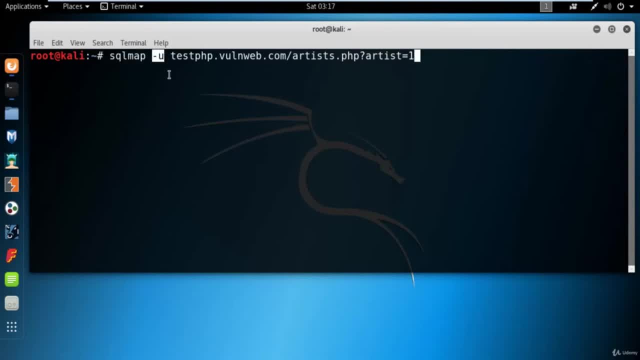 question mark artist equal to one sql map. dash u. after that, type the link of the website and space what you want to find. i want to find the database so you can type dbs- dbs means databases, that's just dbs. to find the databases of this website and hit enter. 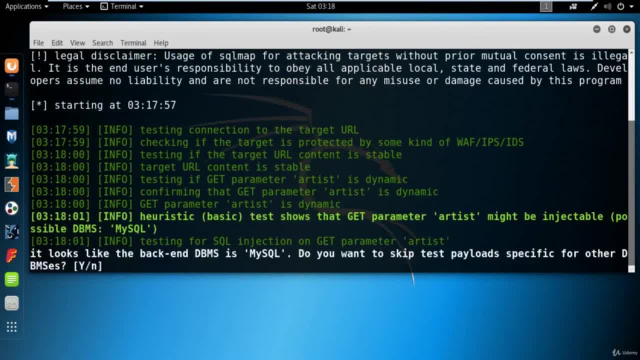 so you can see here that sql map has started and it is asking a question that it looks like the back end is mysql. do you want to skip test payloads, specific for dbmss? if yeah, so what? you will type here, yes or no. it is saying that we have found the database databases regarding mysql. do you want to? 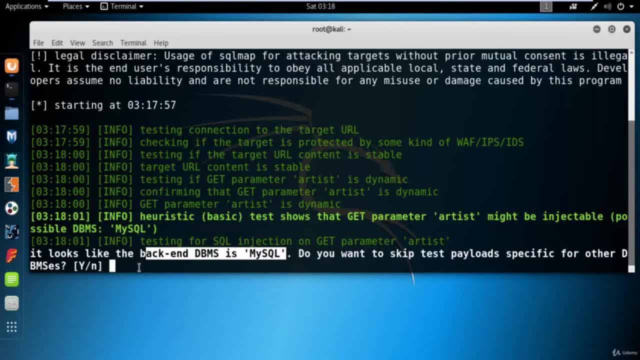 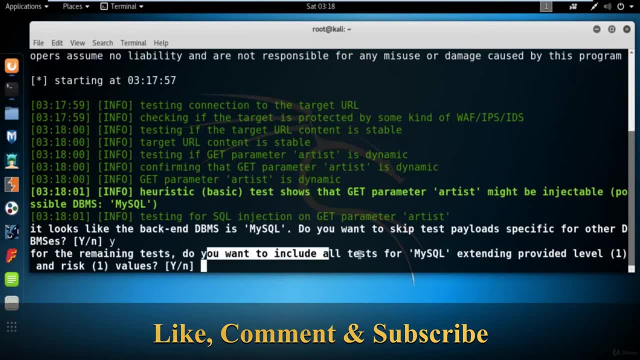 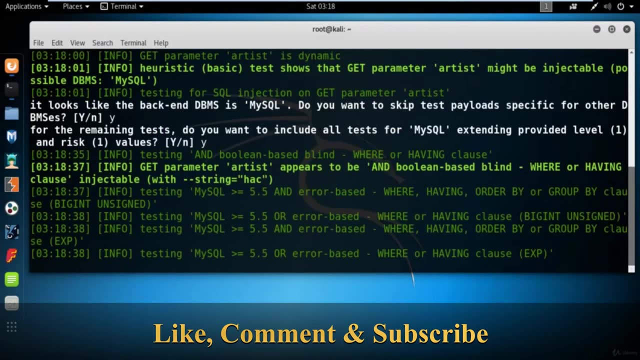 skip. yes, we want to skip because we have already found the database name so you can type y and hit enter. it is saying that for the remaining test, do you want to include all tests for mysql? yes, i want to test and type y and hit enter. now, uh, it is. it will test the web application or the web link. 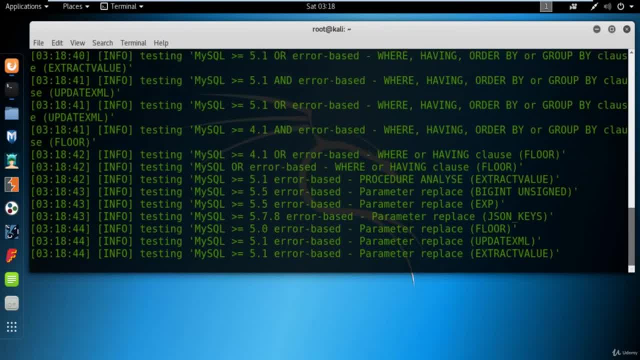 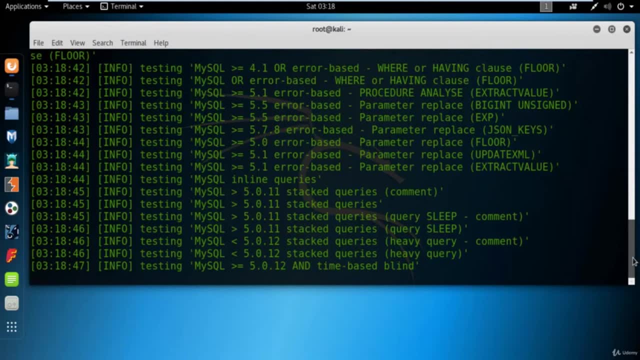 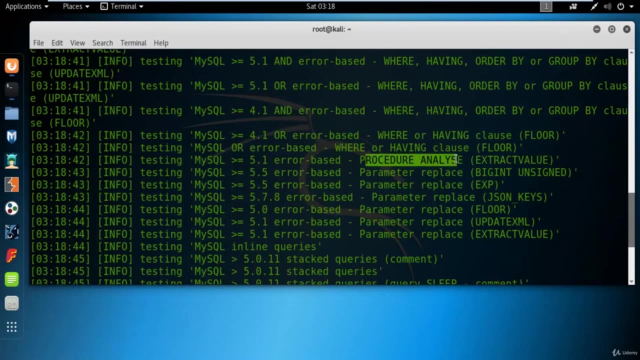 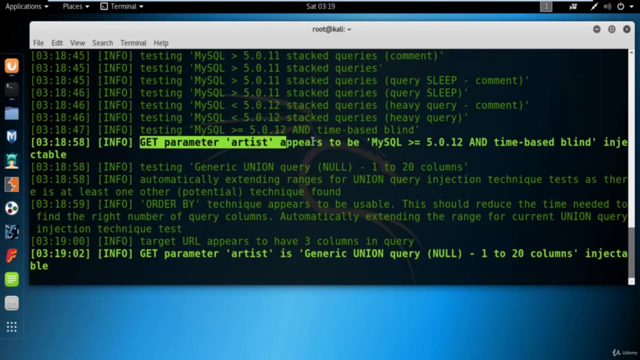 which we have provided, and then it will find out information about the databases in the backend. so you need to just wait, right? you can see here that it is trying. uh, it is attacking on mysql right regarding parameter replay. so procedure analysis right, stack queries- and it is basically attacking on the artist. it is saying that parameter artist appears to be mysql. 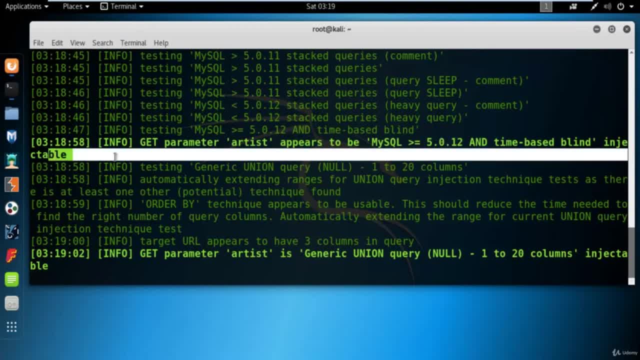 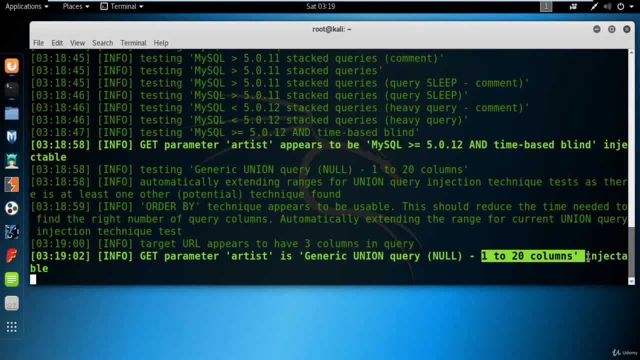 5.0.12 and time based blind injectable. all right, so it is taking some time and you can see here that it is trying on 20 columns and trying to find the number of columns available in the application. so you need to wait and it will find out a single parameter which. 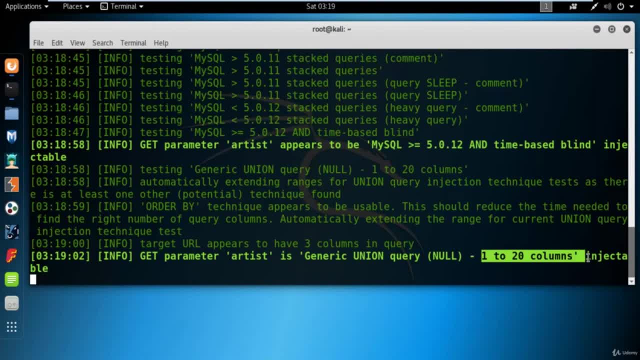 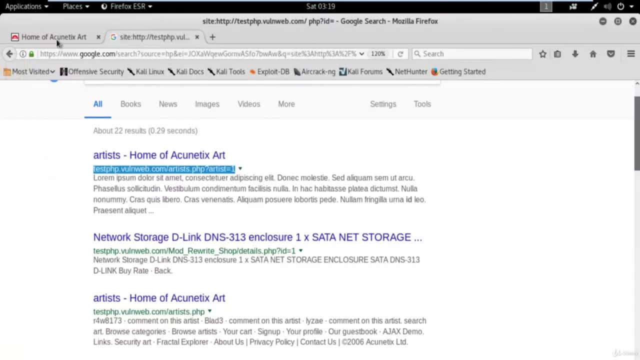 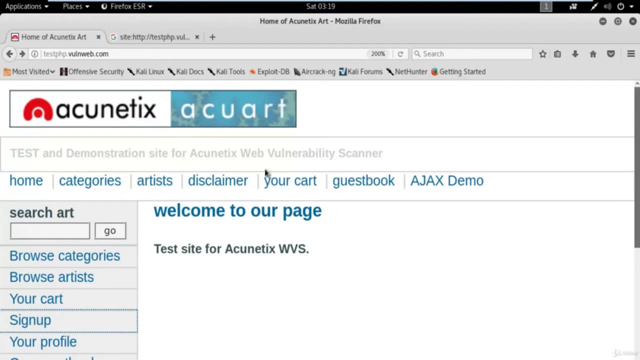 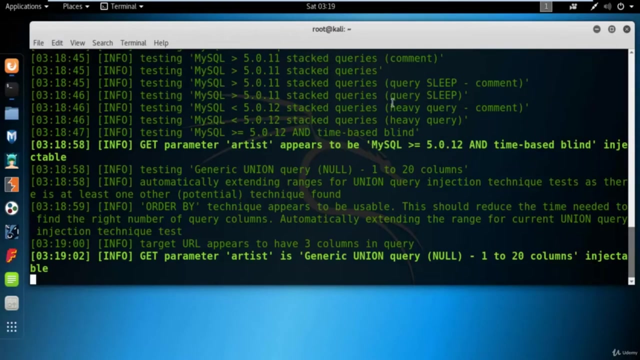 will be vulnerable and we need to use that parameter to uh attack on the website right and then we will able to uh find the basically first the username and password right, and we will be able to change the database information right by using sql injection, so you need to just wait. 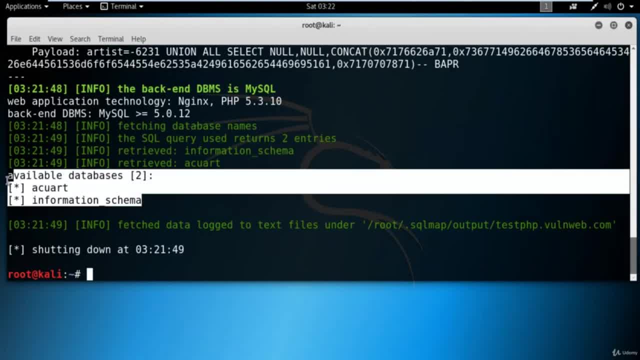 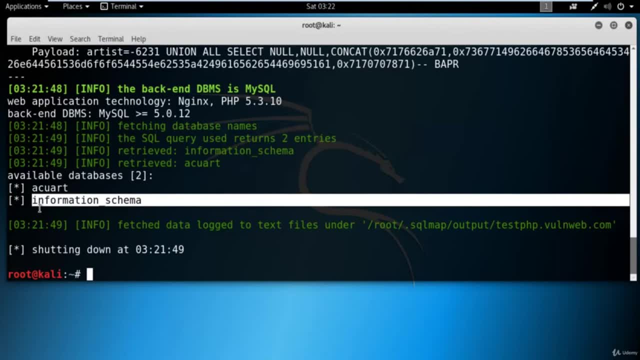 so now you can see on the screen that that we got the two databases here and the first database is accurate and second database is information underscore schema. so basically, information underscore schema is a kind of default database right and we will use accurate database right to find the number of tables. 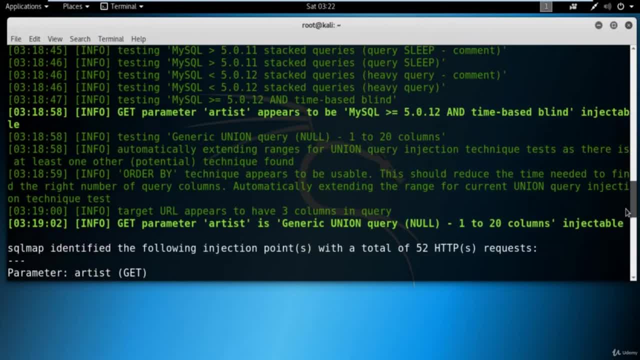 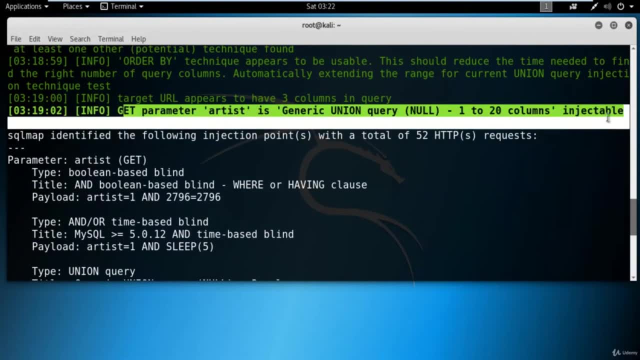 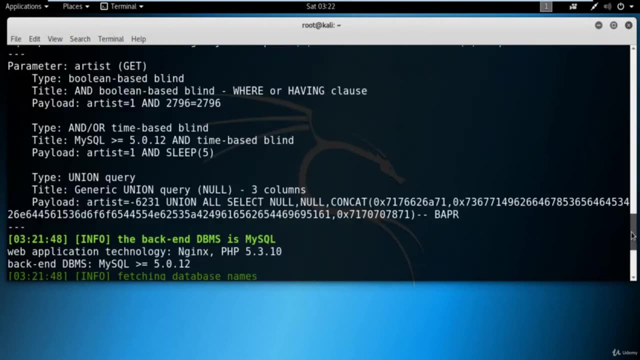 so you can see here that we got the number of databases available here, right, if it just remember one thing: if you get stuck here, right, then please hit enter and it will start it again. all right, so now we are going to use accurate database here to find out information accurate. 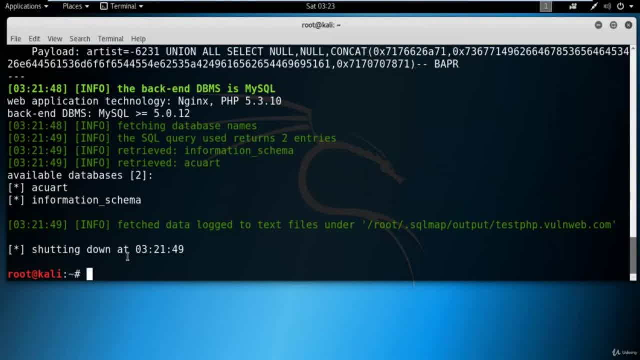 database and now we will try to find the number of tables inside accurate database. so how you can do that, you can simply type sql map space dash u. you need to paste the link space. now you need to specify the database name so database name is accurate. so you can type here: dash, capital d and the name of the database is accurate space, what you need. 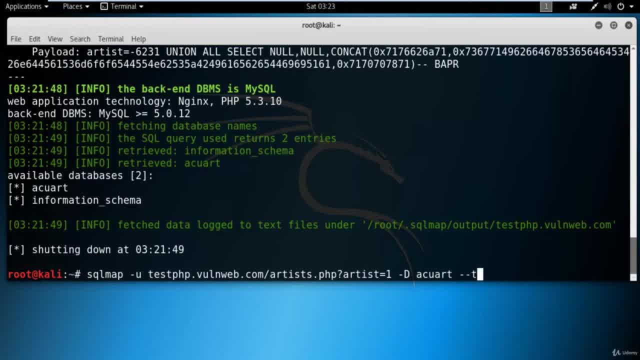 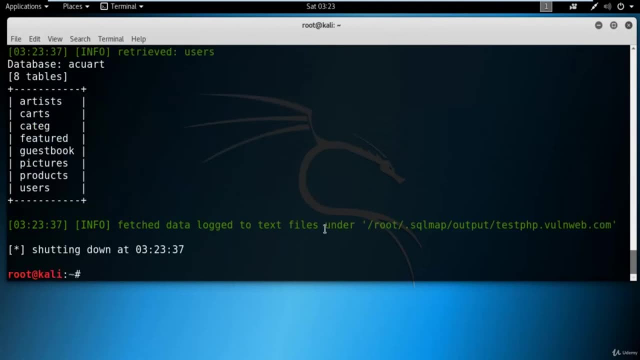 to find. we are finding the number of tables. so you can type here dash, dash tables right and hit enter and you will get the tables inside accurate database. hit enter and you can see that it is retrieving the table names. so here you can see that data inside database acquired there are eight. 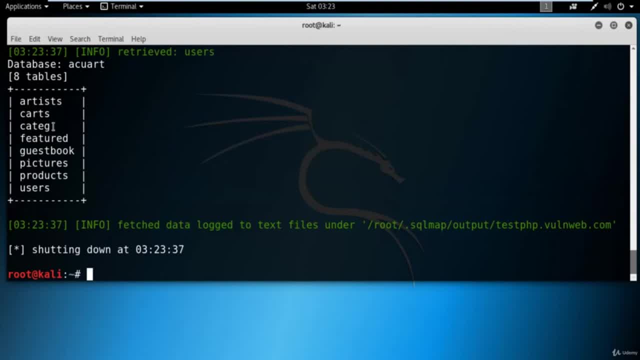 tables and inside eight tables. these are the name of the tables: artists, cards, category users, products, etc. right, so inside a single database there are eight tables, it's it looks like. uh, for example, there is a square right and you are trying to divide that in eight parts so that they are the 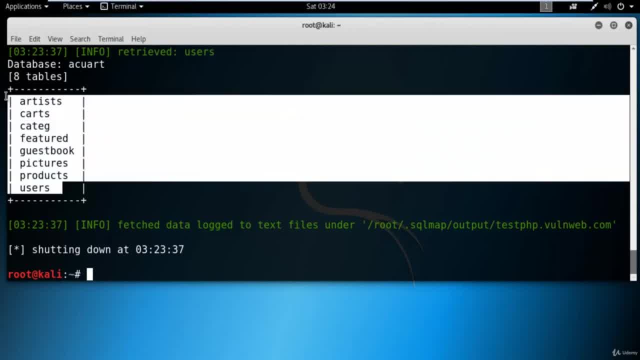 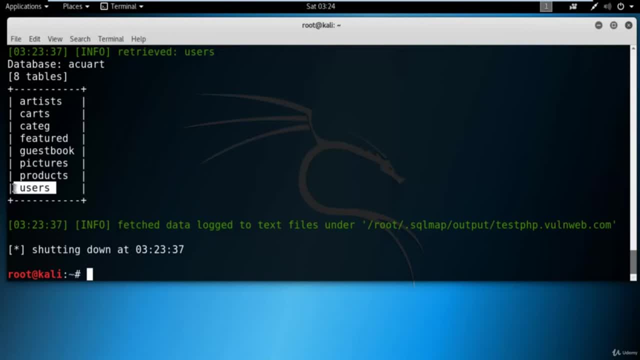 tables in which we need to find out information about the username and passwords. so i think, if i guess, then i think this will be the right table name- i can get information about the usernames, passwords etc. so i will take the user's table name and i will find out the number of columns from this table name. so how we can find the number. 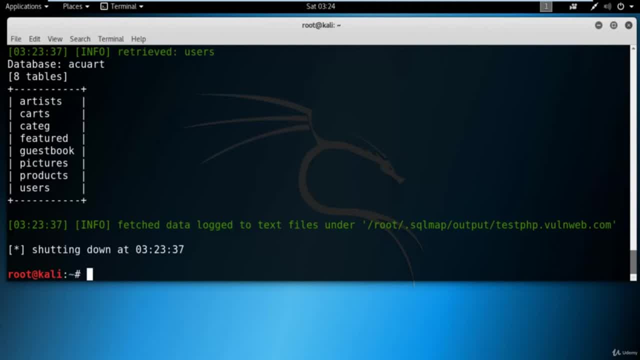 of columns. to find the number of columns you can simply type sql map, space dash u and paste here the link space dash, capital d. you need to type the database name so database name is accurate. that we already found. now we need to specify the table name so that that's capital t. 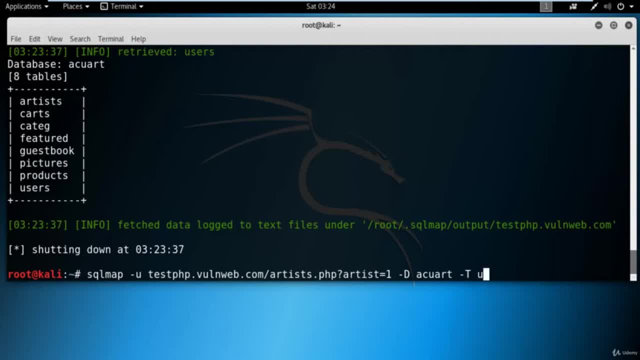 table name is. i'm taking users so you can type here users space and now we are trying to find the column name so we can type column dash columns. all right, so it will provide you the number of columns and the name of the columns from users table right, hit enter. 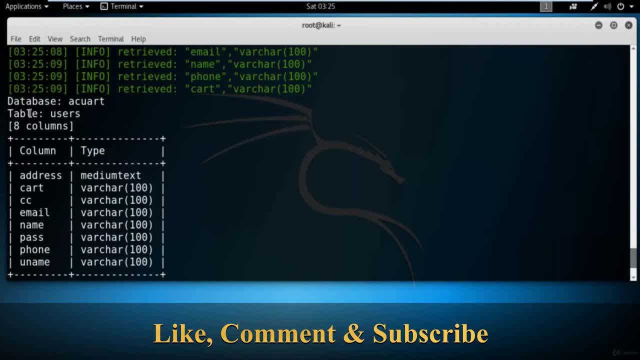 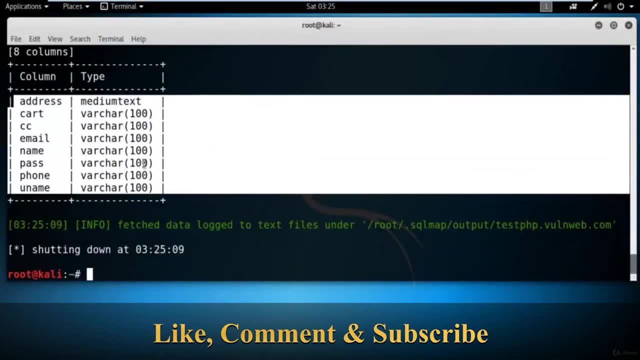 so you can see here that inside database, accurate, there is a table name users. inside table name users there are eight columns available. right, and we have found out eight columns in which you can see there are email ids and password is also available. uname is also available. phone. 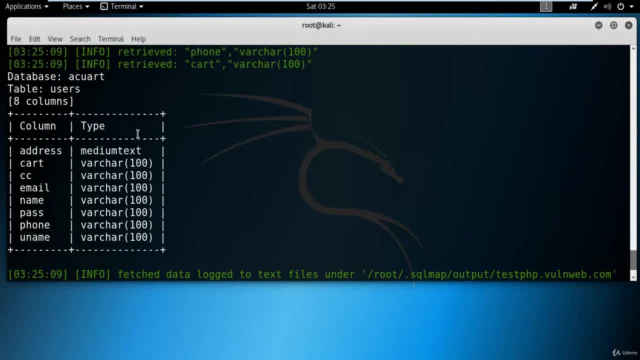 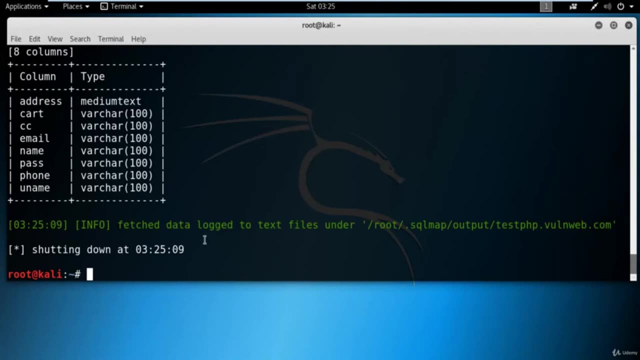 number, address, etc. right now, next task is to find out information about, uh, first of all, uname. uname is, i think, username and pass is, i think, password, i'm just guessing right. so, uh, let's find out information about the? u name first of all, so to get username information. 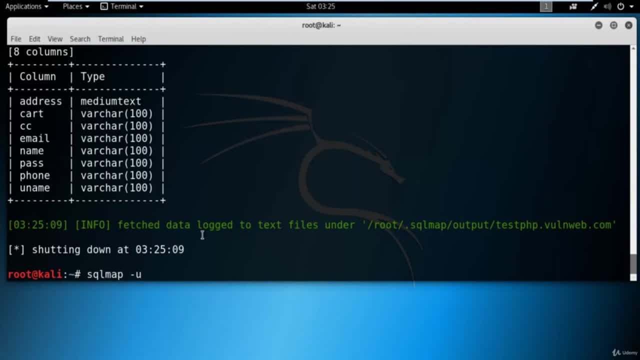 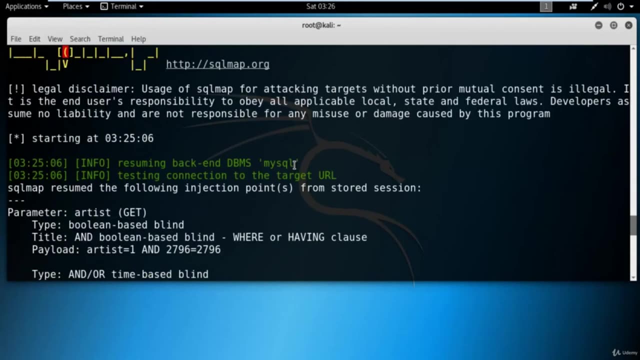 you can type sql map dash u, paste here the link space dash capital d and you need to specify the name of the database which is acquired: dash capital t. you need to specify the table name. so i think the table name was users, right inside users table name. 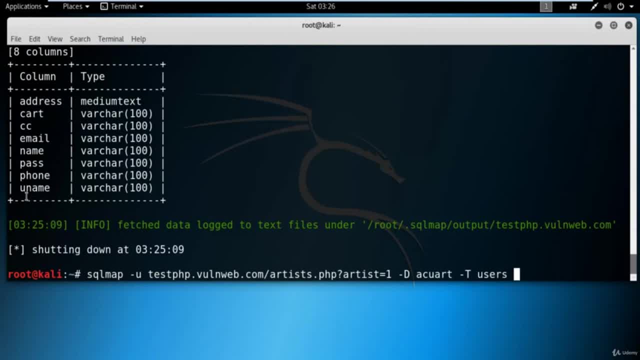 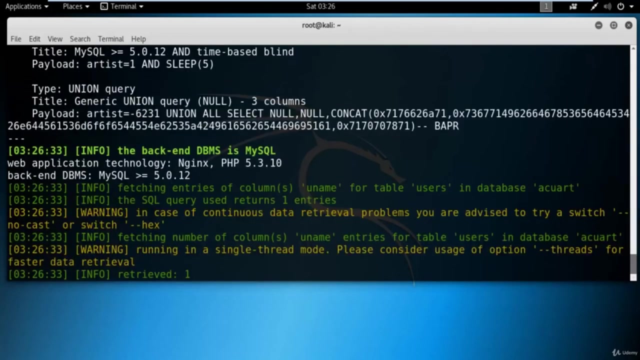 we are trying to find the column. so the column name is uname. you can type dash, capital c and uname, right space dash dash dump. so finally you need to type dash dash dump to extract the information about username from these tables. right hit enter. so there is only one column. i think it is showing just one here. 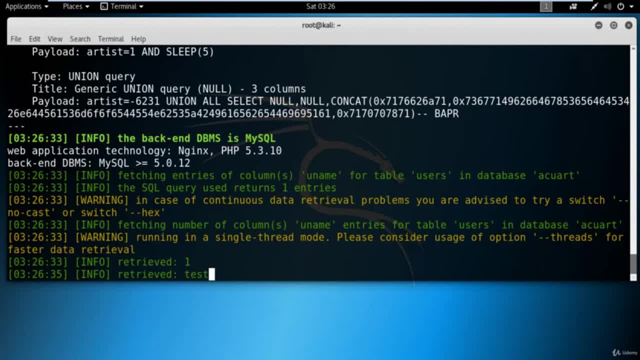 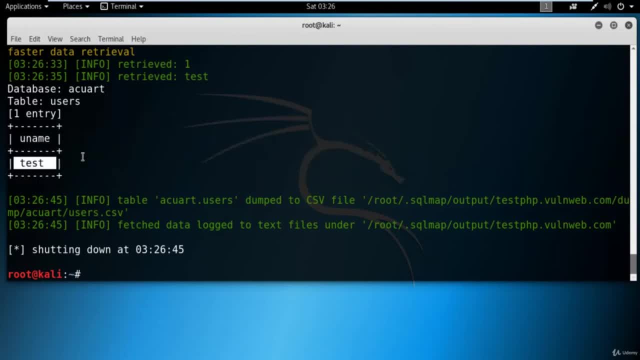 and it is showing us the username t-e-s-t. i think yeah, so you can see here. that is, that it has provided us the username information. username is test. similarly, we can find information about the password. so you can type here: just click here and click on your upper arrow of your keyboard. 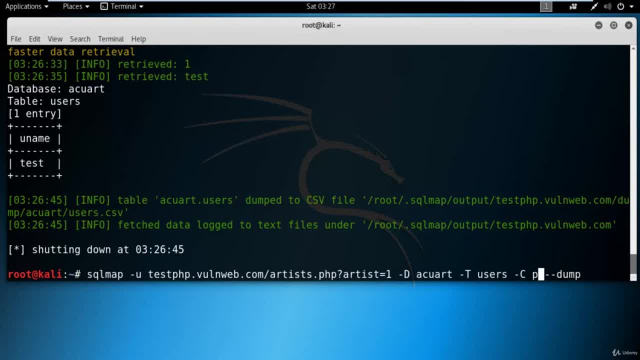 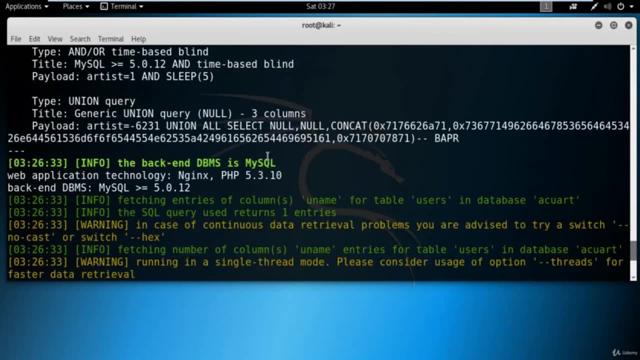 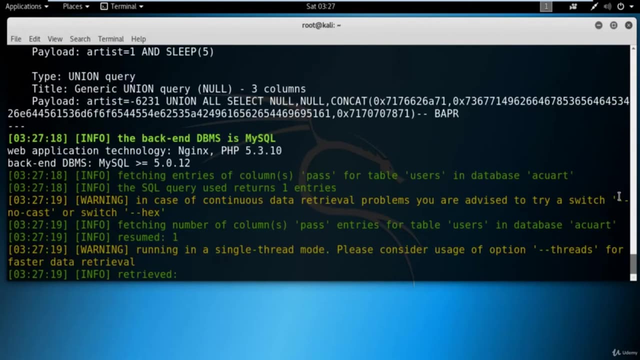 right and just replace this uname with p-a-w-s, because, uh, there is another column available there. you can see that the name of the column is p-a-w-s, so we are going to find out information about password as well. and hit enter. now it is retrieving the password from the database. 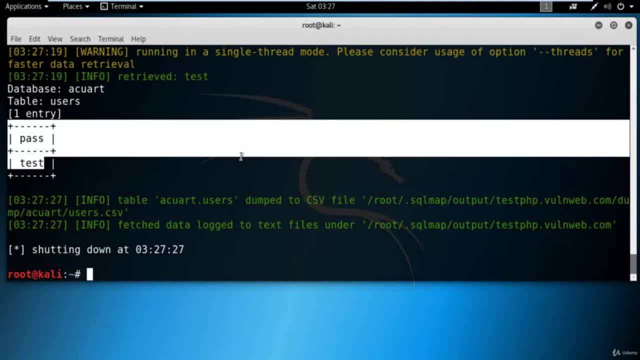 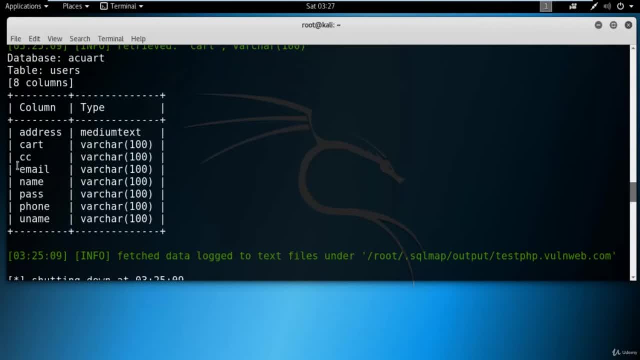 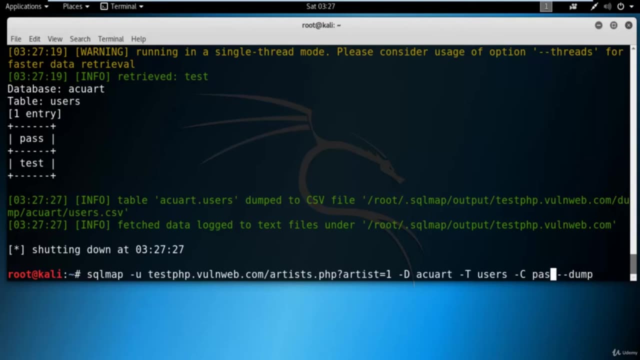 right and i think you can see on the screen that the password is also test. so username is test as well as password is test. you can also get information about other information, like email ids. so what you can do, click here, click on up arrow to get the command again and you can. 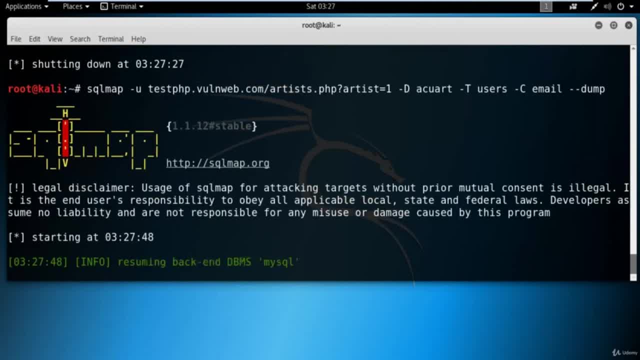 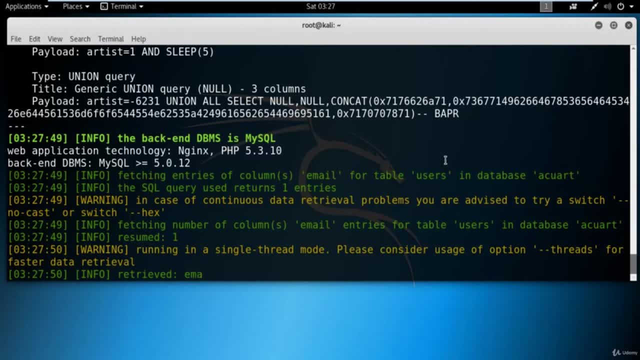 type email here to get information about email. so extracting email ids whatever. inside that, slowly, slowly it is taking one character at a time. you can see here that it is extracting the email id whatever. basically, it is a sample website, right? so that's why all the information 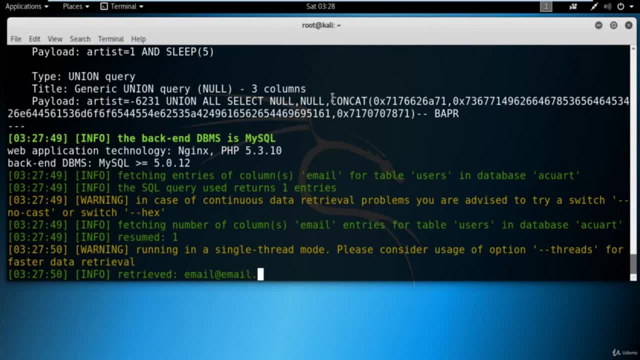 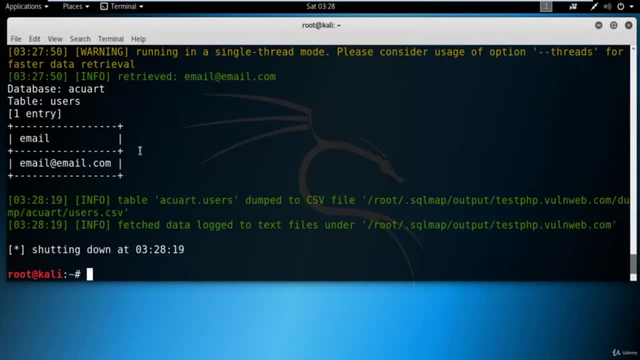 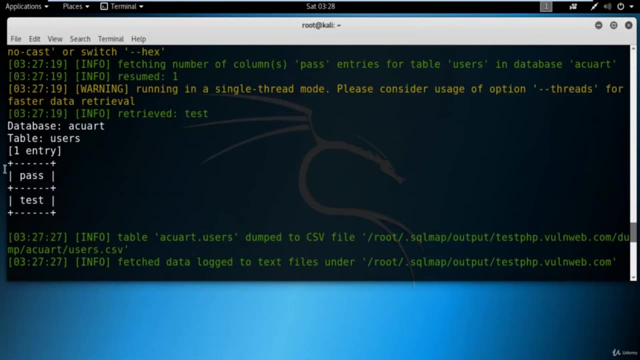 available inside the database is also sample, so you can see here on the screen that it is trying to extract the email ids and here it is. so this is kind of email id available inside the database. great, so we got the username right. this is the password test and this is the username test. 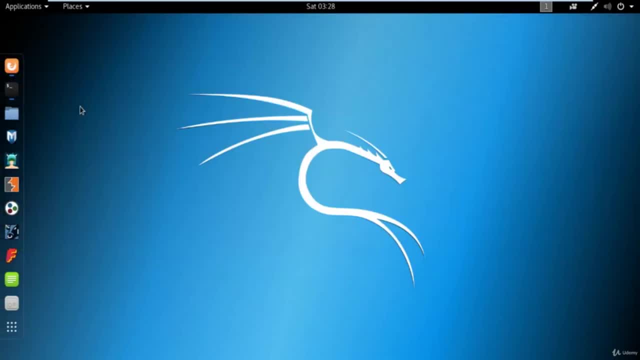 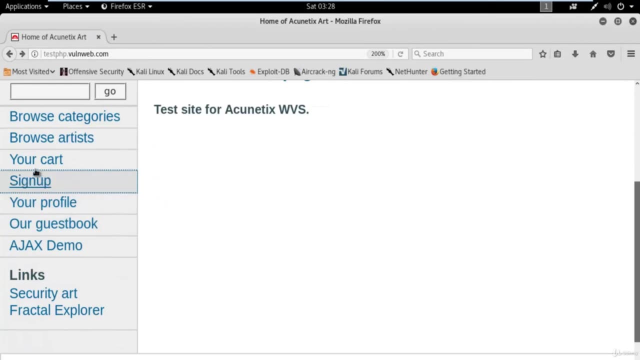 available. so what we can do here just minimize the data. so this is the password test and this is the username test available. so what we can do here, just minimize this. open the website and in that website you can see on the left hand side there is a button sign. 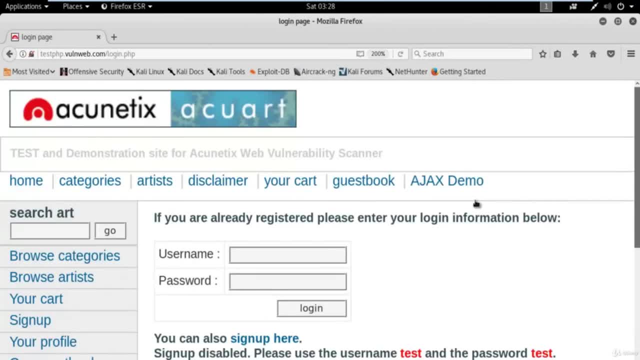 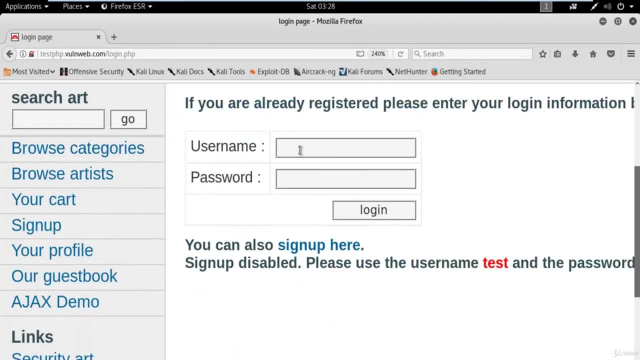 up button here. so click on that and on that sign up button you can see there is a username and password. can you see here? yeah, this is the username and password panel. right, so we got the username. the username is test and the password is also test. you can click on login. 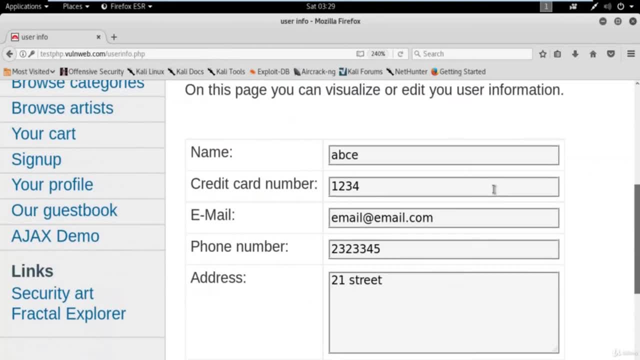 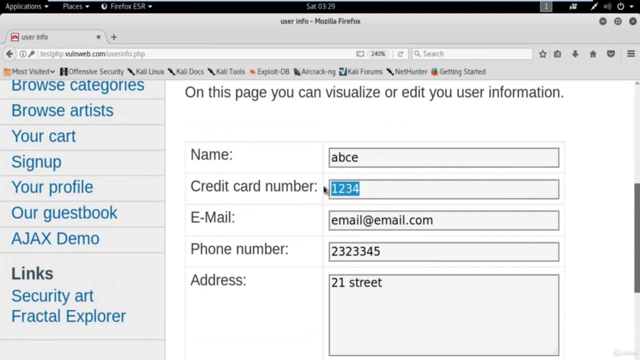 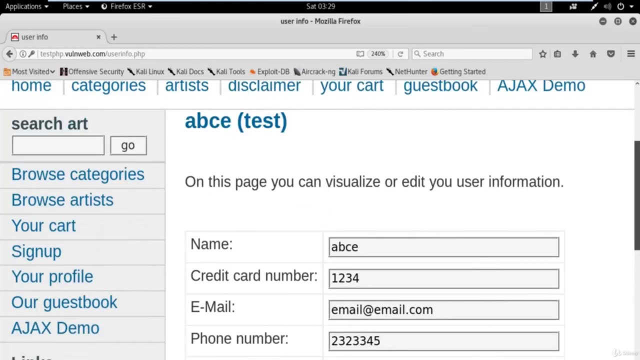 and you can see here that you are able to get information about the database here. right, you can see the name, you can see if there is any credit card number, if there is an email id, if there is any phone number address, you can also update the information from this database. so to 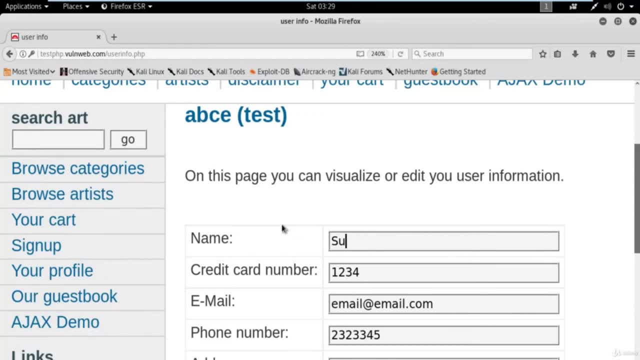 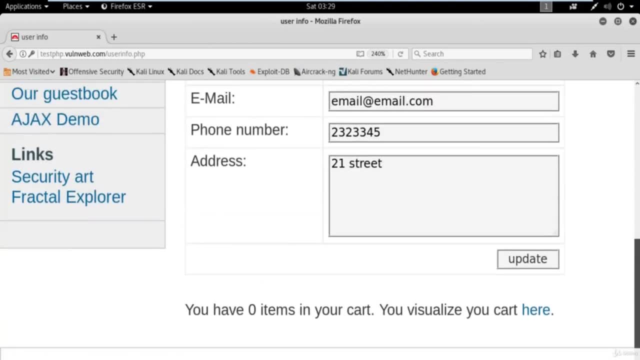 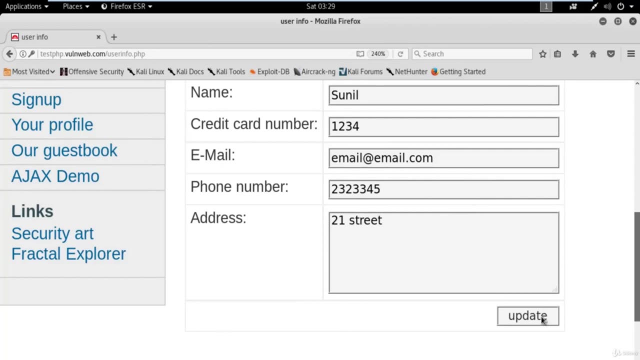 update the database. you can simply remove the name. let me type my name right and let me click on update. please don't put your original information here. original information like don't put your phone numbers or email id address, credit card number, right so because this is visible to all, of all the type, all kind of hackers. so click on update, right it. 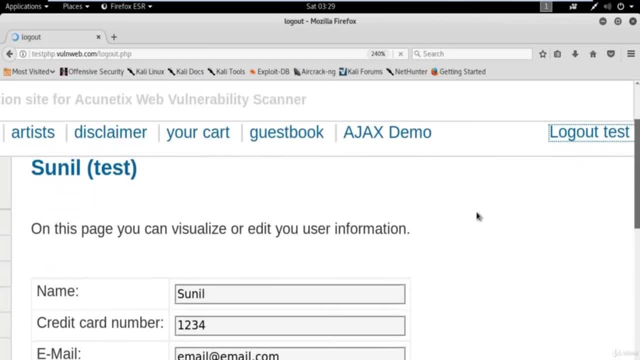 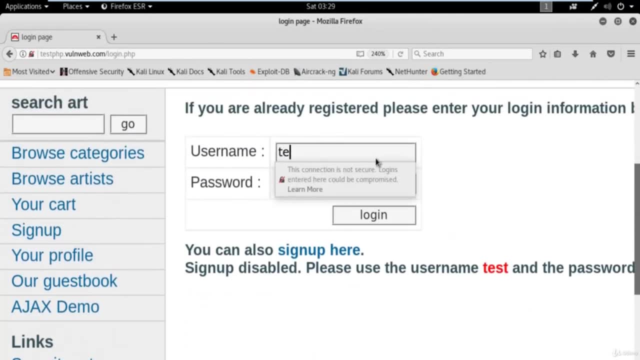 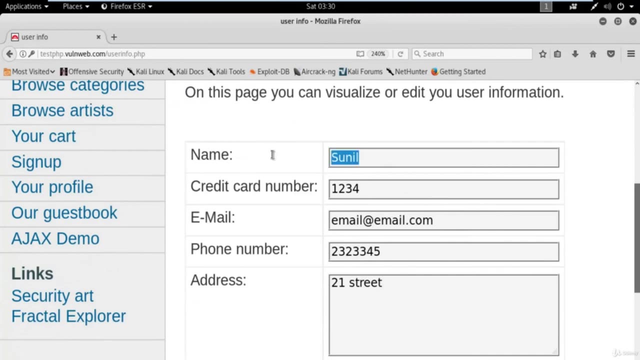 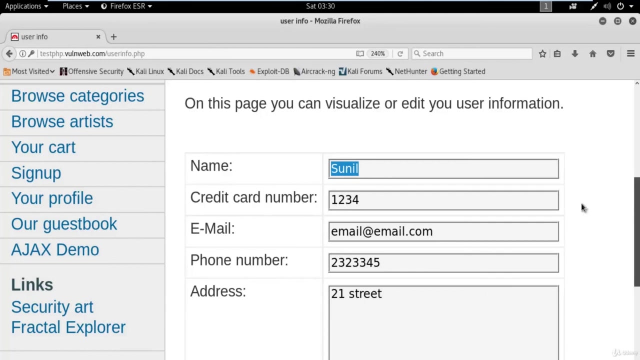 has been updated. let me log out, let me log in again, let me click on sign up and if I type here test and test and if i click on login, then you can see here that my name has been updated in that database. basically, i have updated their database and i have put my entries inside. it got my point, so you.